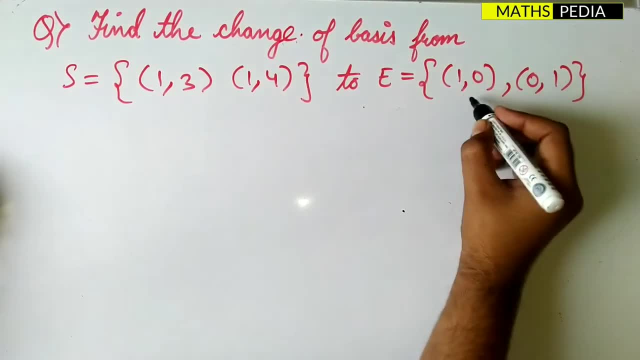 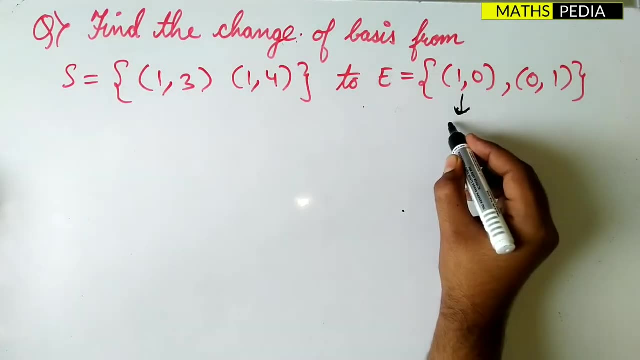 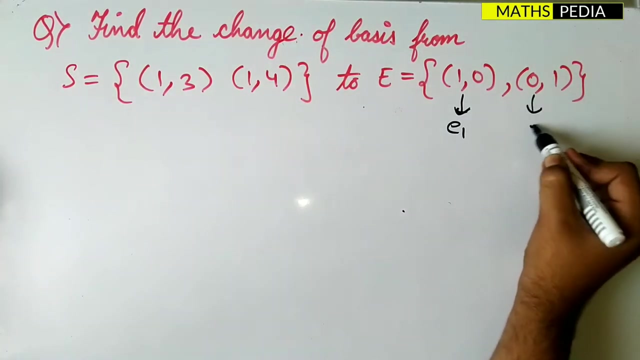 So it will be in the form of linear combination That I will teach you. So to where, From S to E, whatever is there to. so I can take it this one as this is nothing but what change of basis? this is standard basis. It is nothing but E1,. this will be E2, standard basis. 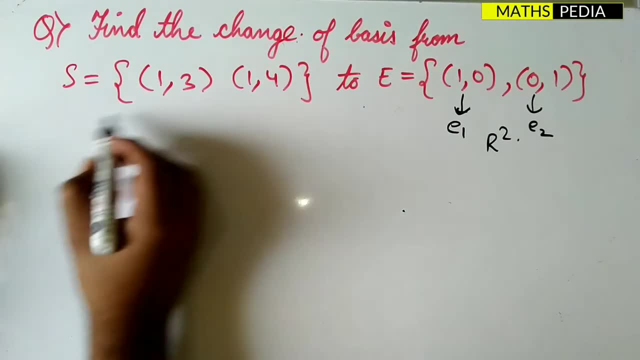 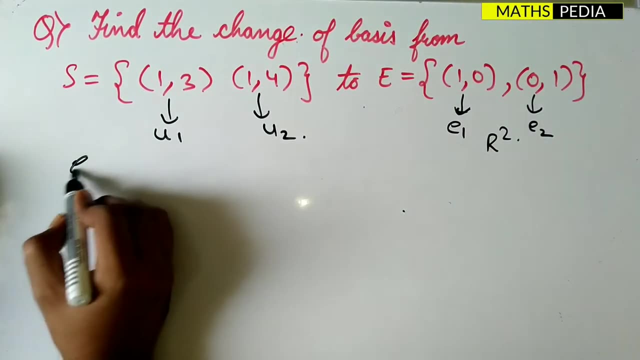 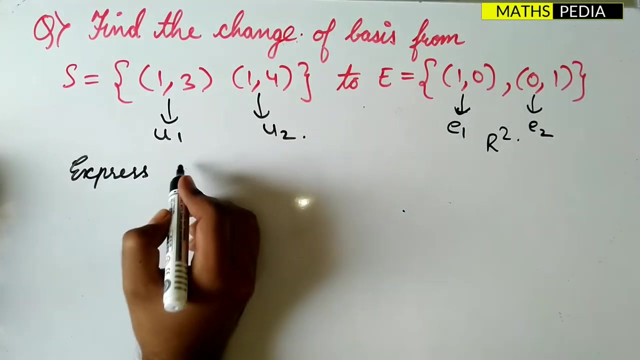 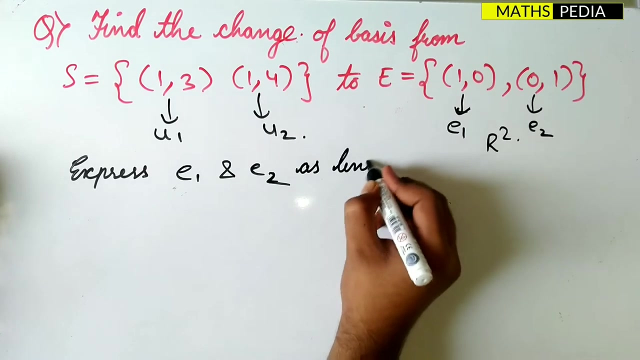 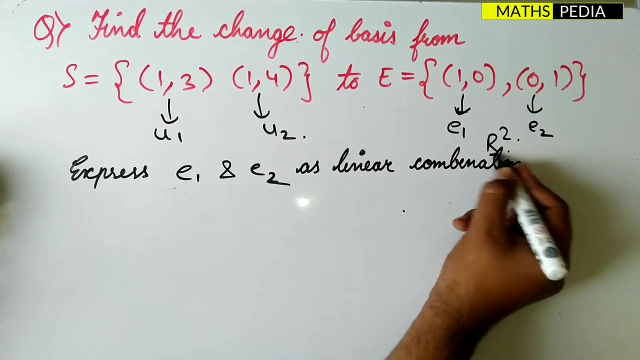 Okay, standard basis Now. so I will assume that this one to be U1 and this one to be U2.. Now the first step is that you have to express, express what, whatever is there- E1 and E2, that I have to express as linear combination, linear combination of U1 and U2.. 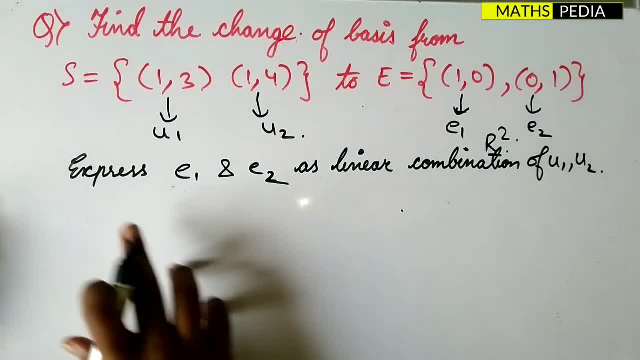 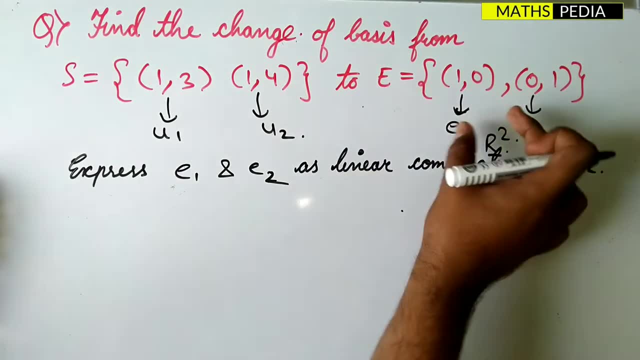 Observe here carefully. what I am doing is that Expressing E1 and E2.. Why E1 and E2? Because it is a change from S to E. So whatever E is there, that you have to take E1 and E2 as linear combination. Now how to express this? 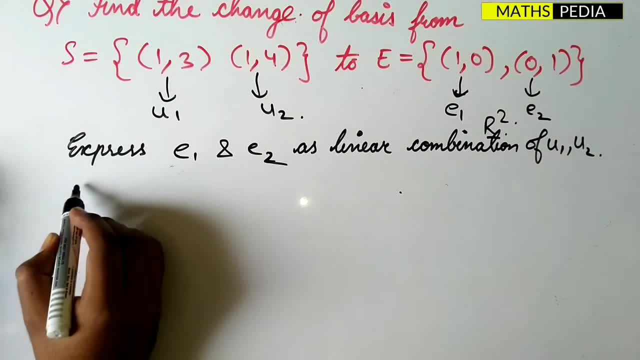 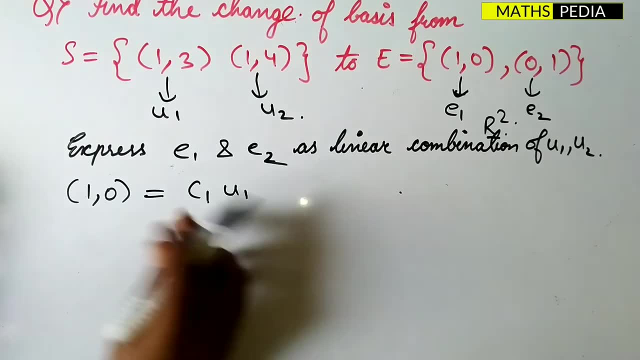 So observe carefully: E1 is given as 1, 0. So I have to write it in the form of C1 into U1, because U1 is there in the S, plus C2 into U2.. Okay, so what is C1?? 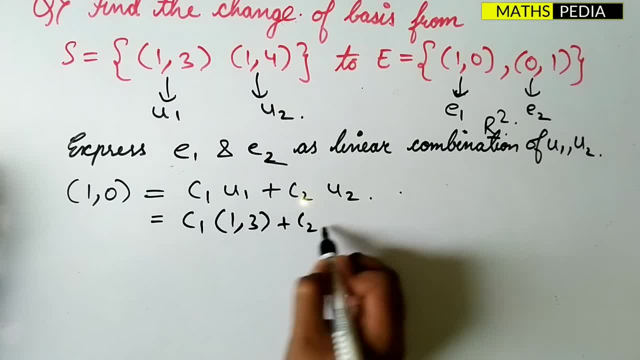 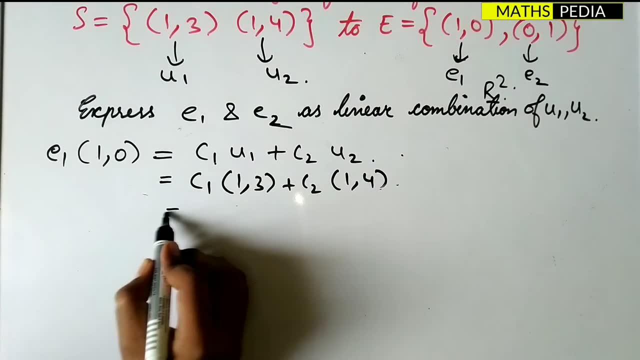 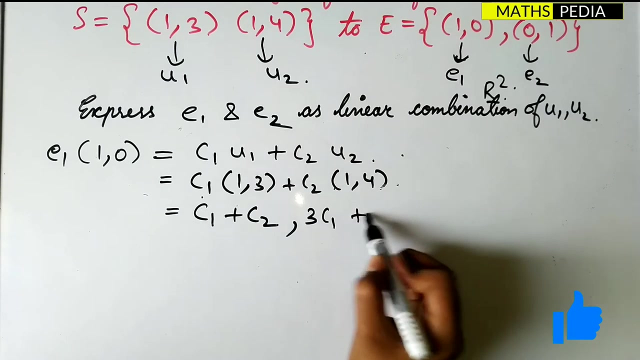 E1 is given as it is, U1 is given 1, 3 plus C2 into. U2 is given as 1, 4.. Now I have to simplify this part and find out C1 as well as C2.. So this will be C1 plus this one, C2, 3C1 plus 4C2.. 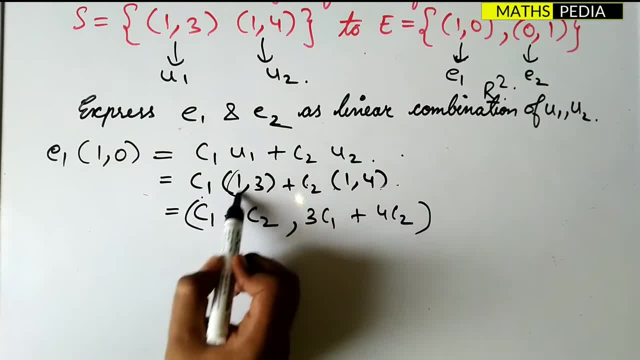 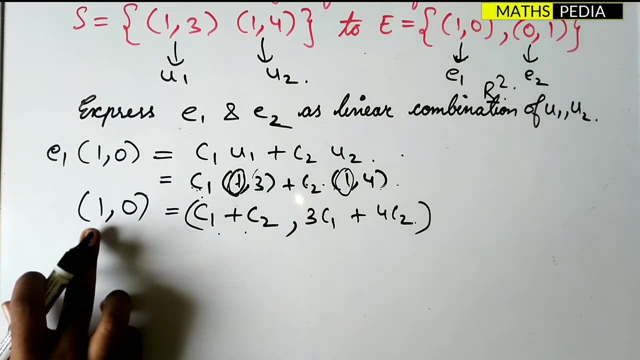 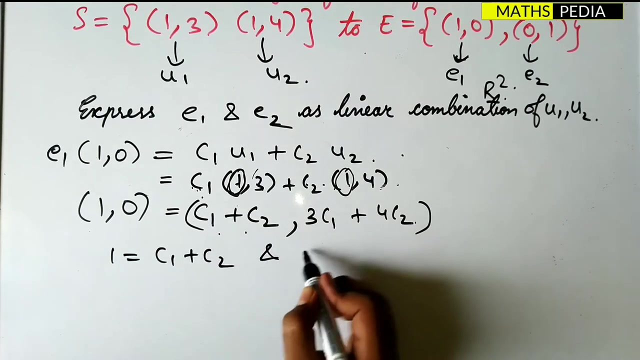 Okay, I hope you got it For this one. see the first part. here- also first part- you have to write C1, C2.. Then, second part, you have to choose 3C1, 4C2.. Okay, this I have written Now, which will be equal to 1, 0. See here: 1 will be equal to this part, 0 will be equal to this part. So 1 is equal to C1 plus C2 and 0 is equal to 3C1 plus 4C2.. 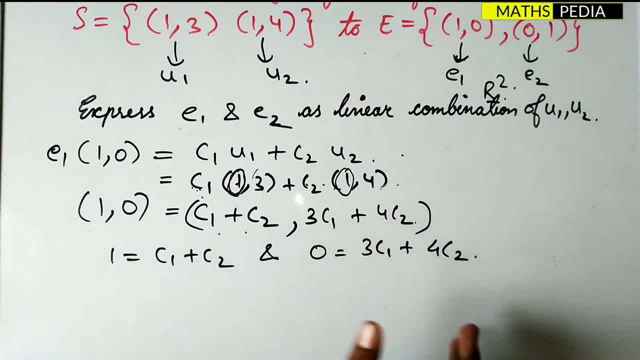 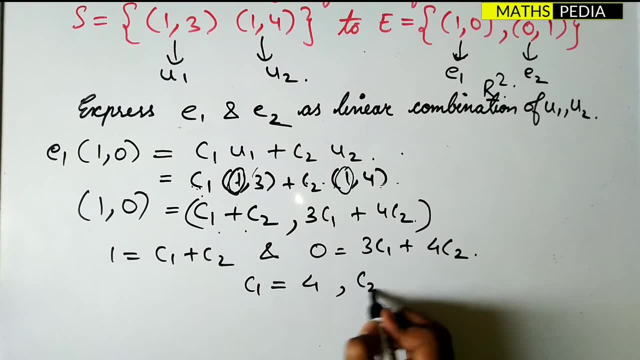 Now I have to solve these two equations And find out the answer. You can just calculate in the calculator and just get the value. I will get it as C1 as 4 and C2 is equal to minus 3.. Okay, C1, I got it. C2 also, I got it. 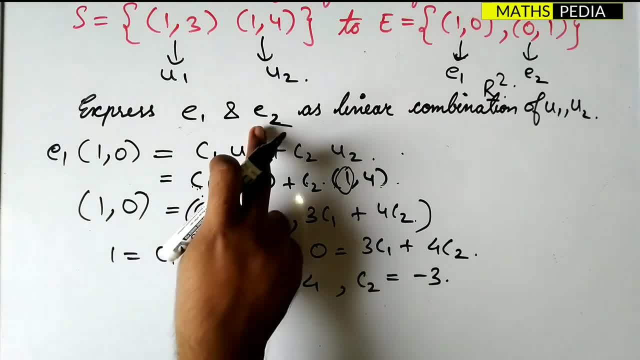 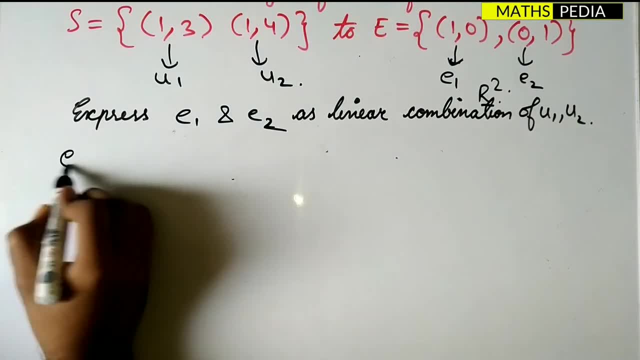 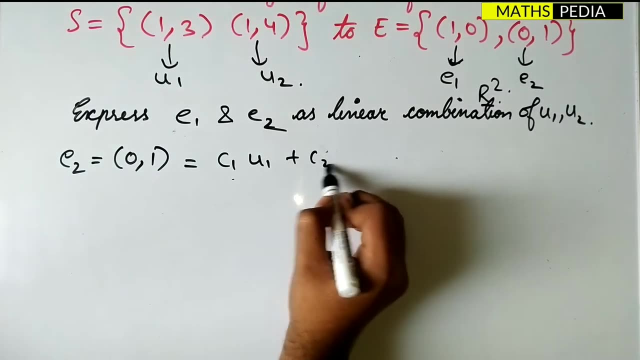 Now next thing: I have to express E2 also as linear combination of both U1 and U2.. E2 I will take which is equal to 0, 1 linear combination I have to express That will be C1 into U1 plus C2 into U2.. Same thing, But the difference is LHS will be changed. 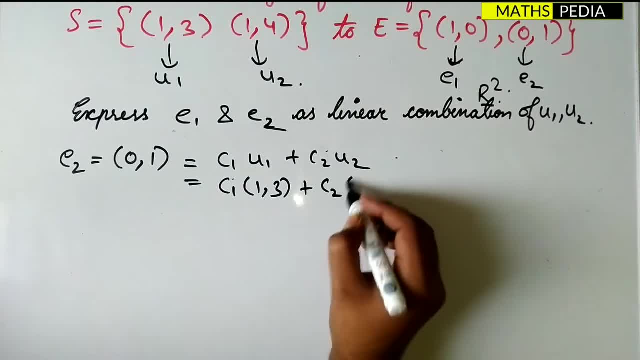 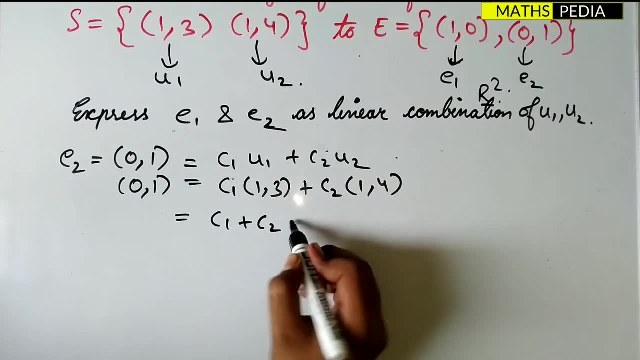 C1 into U1,, it is 1, 3 plus C2 into 1, 4, which is equal to 0, 1, and it is equal to C1 plus C2, comma 3C1 plus 3C- sorry, 4C2.. 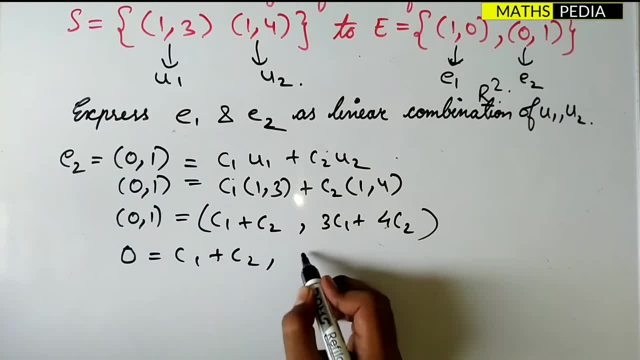 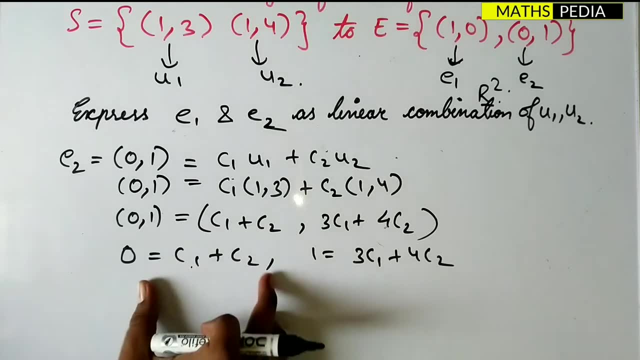 Therefore, 0 is equal to C1 plus C2.. And 1 is equal to 3C1 plus 4C2.. So therefore, C1 will be equal to minus this two equation. I have to take and just solve it in order to get the value. 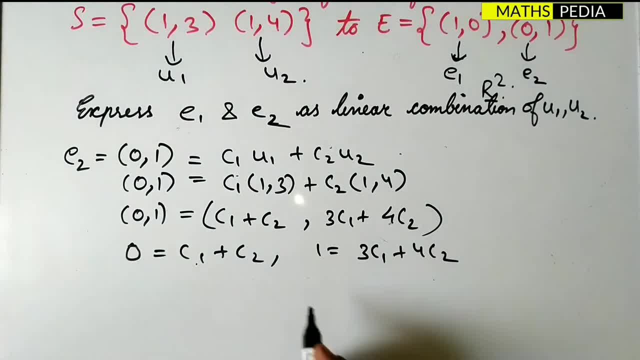 So how I can get the value. Therefore, after solving this, what you will get? C1, you will get it as minus 1, and C2, you will get it as plus 1.. So, from both the cases, I got C1.. 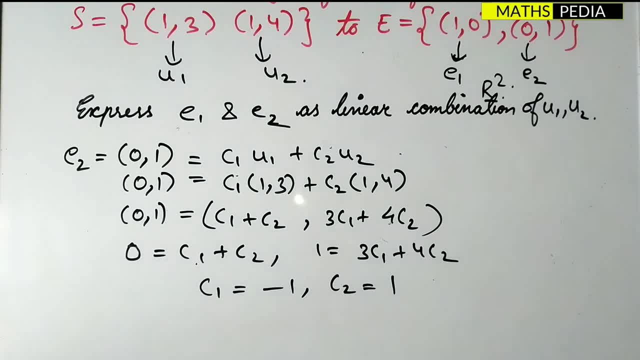 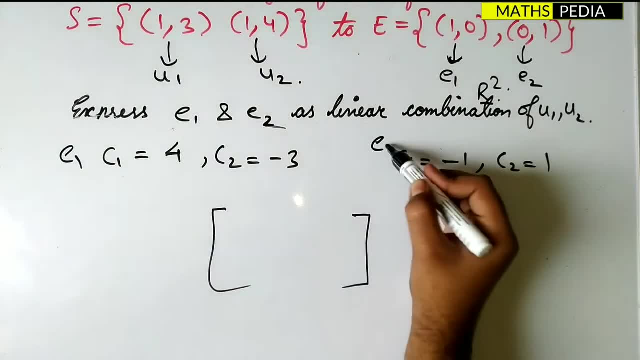 As well as C2.. Now I have to arrange it in a matrix form, So always remember this When you arrange in a matrix form. this is the first case, E1,. this is the second case, E2.. Okay, first one, second one. 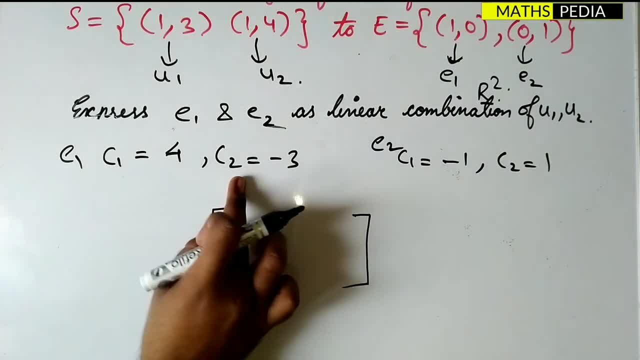 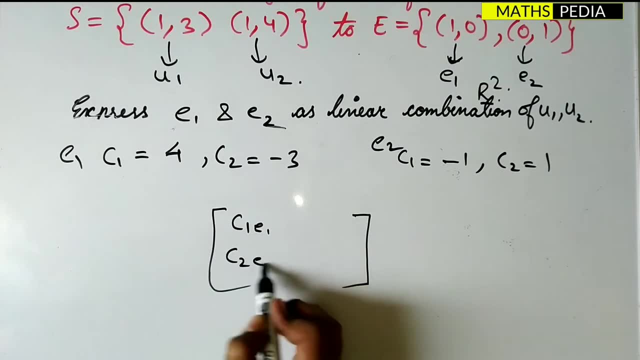 So first one, whatever you got, C1 and C2, you have to arrange in column. That is C1, I can write it as E, E1, something C2, E2,, sorry, E1.. For the E1 case I have to arrange in column. 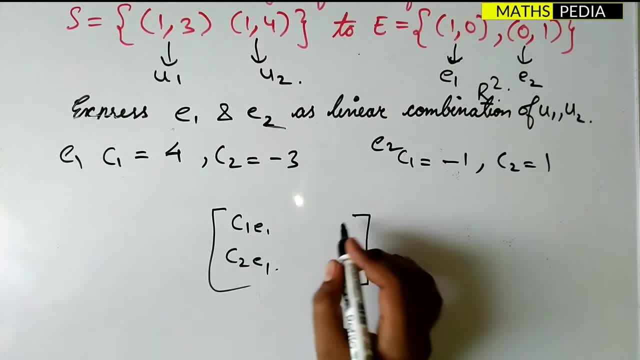 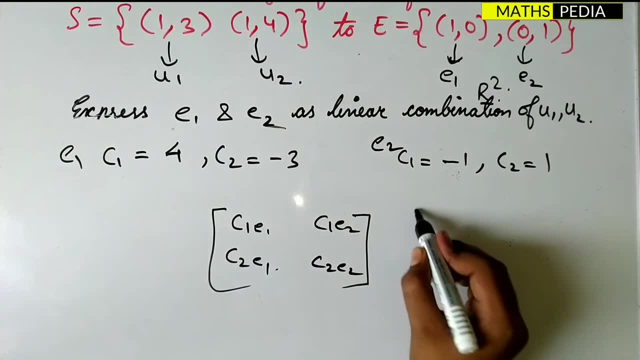 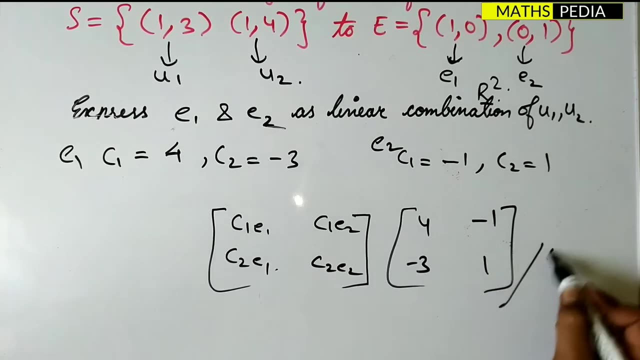 Next, For this case also column wise, second column, That will be C1, E2 and C2, E2.. Okay, So this becomes 4 minus 3 and minus 1 and 1.. So this will be the final answer. 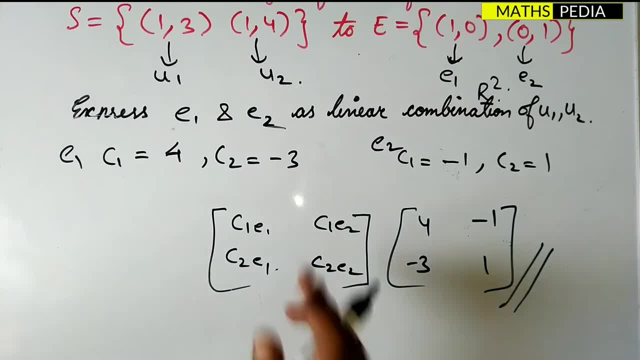 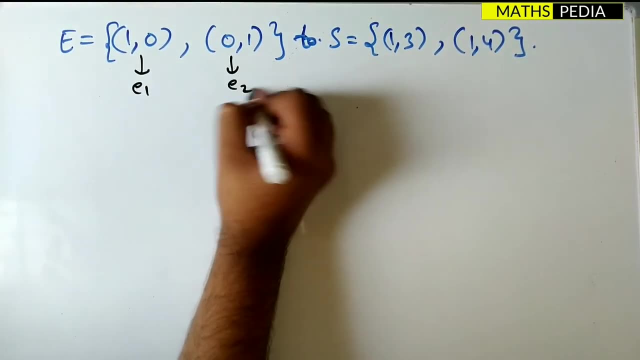 This is not multiplication, this same thing. Okay, this will be the final answer. Now we will try to analyze how we can convert, how we can find the change of basis from E to S. So for this, what I need to do this is nothing but E1, standard basis, E2, this one is U1, it will remain as it is. 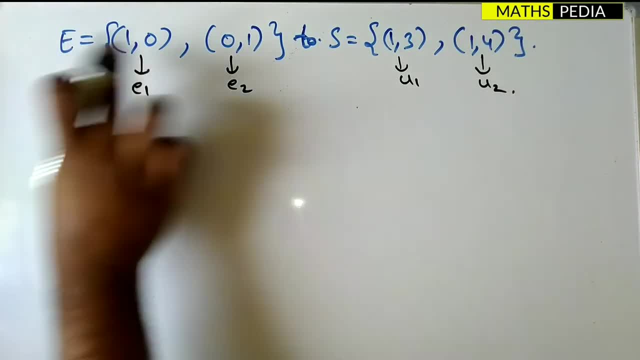 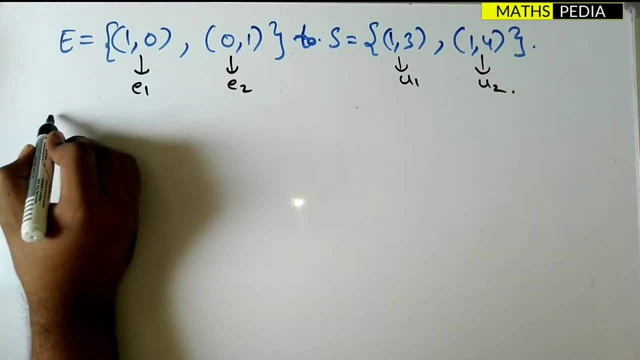 Okay, U2, U1 and U2.. Now it is from E to S, So whatever is there, U1, U2, I have to express this, this two, as so it will change. So express U1 and U2 as linear combination. 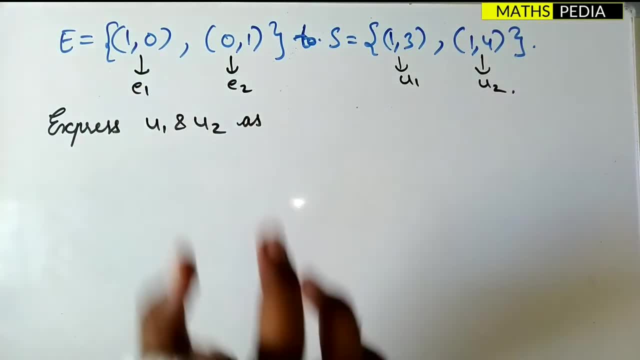 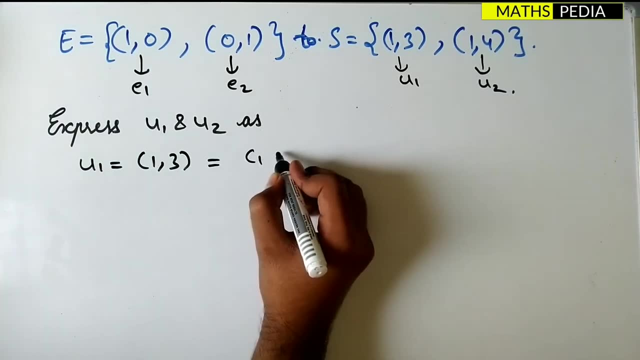 Okay, Okay, Linear combination of E1 and E2.. Now I have to take U1, which is equal to 1, 3. I have to write it in form of C1 into now. it will change it into E1, plus C2 into E2.. 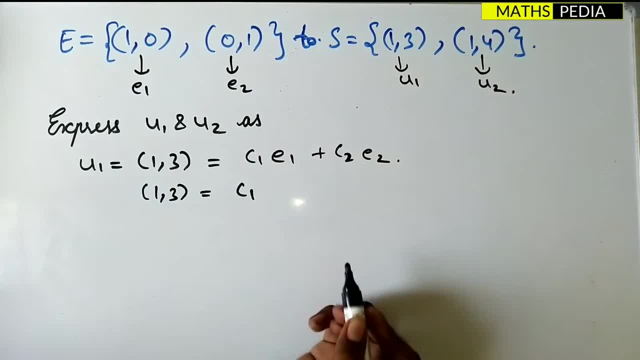 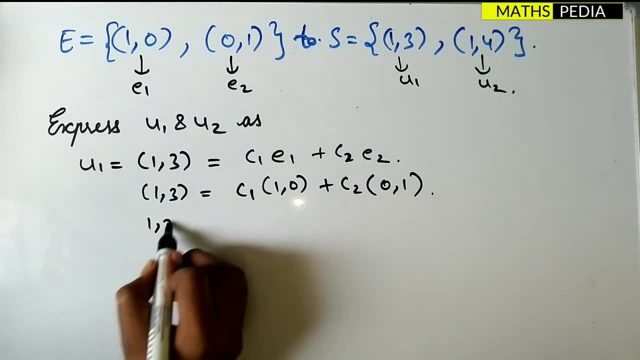 So 1, 3 is equal to what is C1?? C1 will remain as it is. E1 is 1, 0 plus C2 into E2 is 0, 1.. So 1, 3 is equal to C1.. 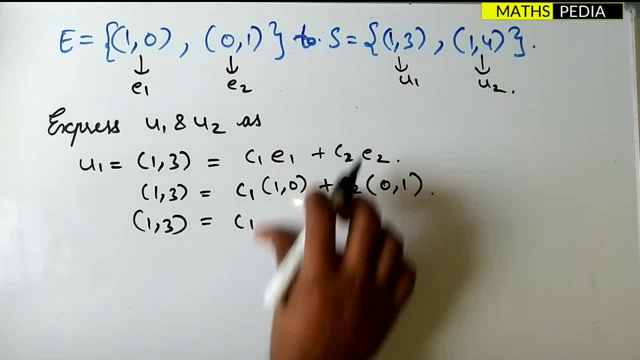 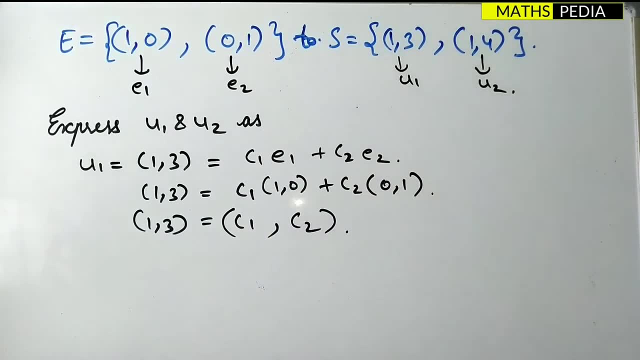 Next, I have to express U2. as well as U2, I have to express: U2 is 1, 4, which is equal to C1 into E1 plus C2 into E2.. So which will be equal to C1 into 1, 0 plus C2 into 0, 1.. 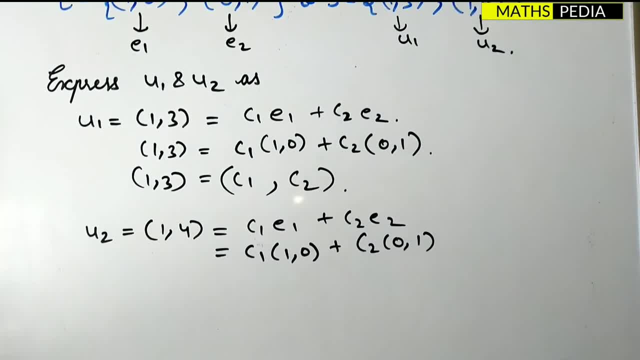 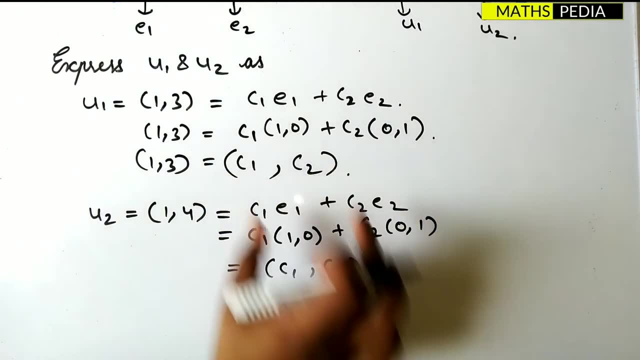 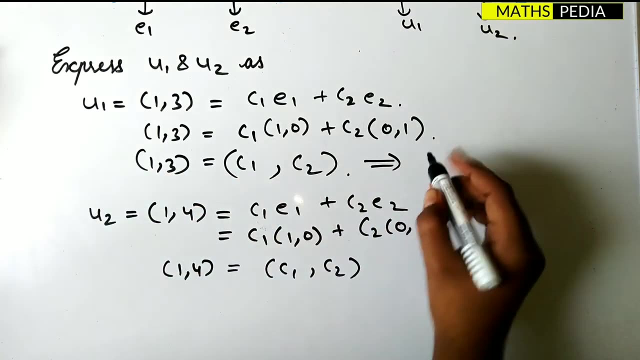 You can directly write this part itself, So no need to do this much of steps. You can avoid that. So, which will be equal to C1 comma C2.. This RHS will remain as it is, Okay. Only the LHS changes 1 comma 4.. So from this I can write: 1 is equal to C1.. Sorry, C1.. Ah, yeah, 1 equal to C1.. 3 is equal to C2.. Correct.